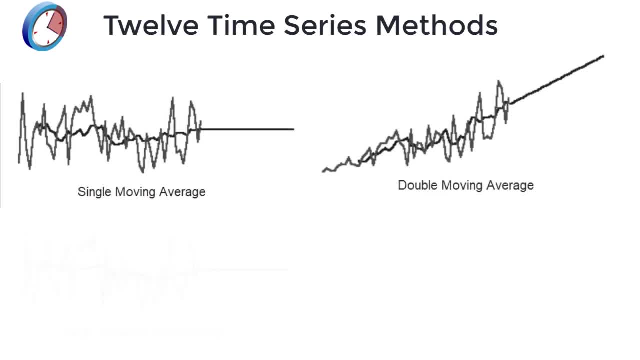 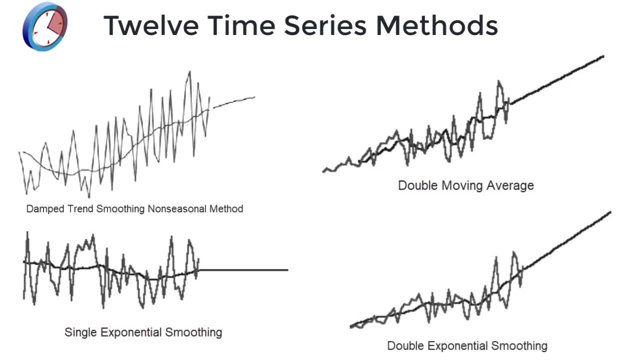 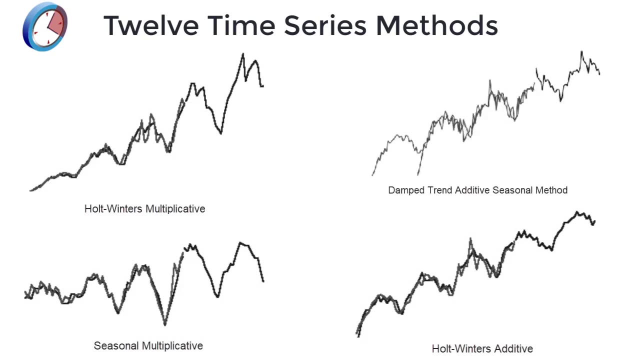 Single Moving Average. Double Moving Average. Single Exponential Smoothing. Double Exponential Smoothing- Damped Trend Smoothing- Non-Seasonal Method- Seasonal Additive Seasonal Multiplicative Holt- Winters- Additive Holt- Winters- Multiplicative Damped Trend Additive Seasonal Method. 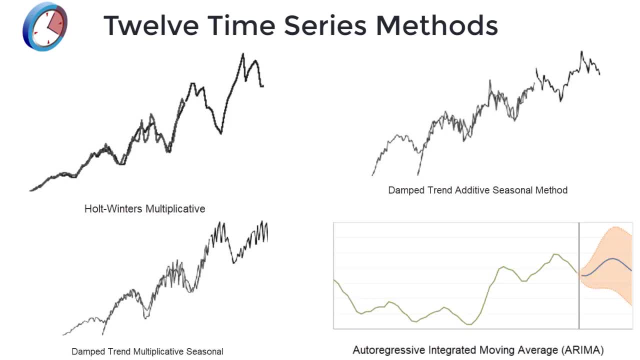 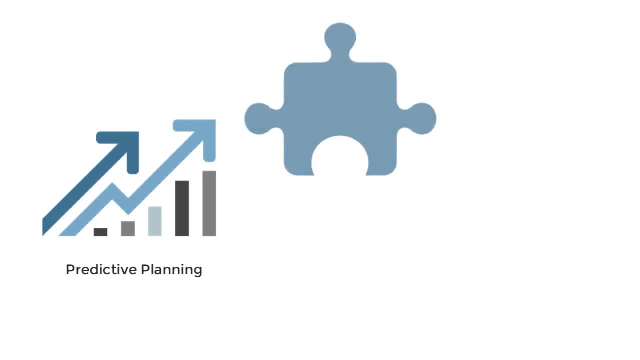 Damped Trend Multiplicative Seasonal Method. Seasonal Multiplicative Seasonal Method. Auto-Regressive, Integrative Moving Average. Predictive Planning runs each method on the data and calculates a mathematical measure of goodness of fit. The method with the best goodness of fit is the one used to give the most accurate prediction. 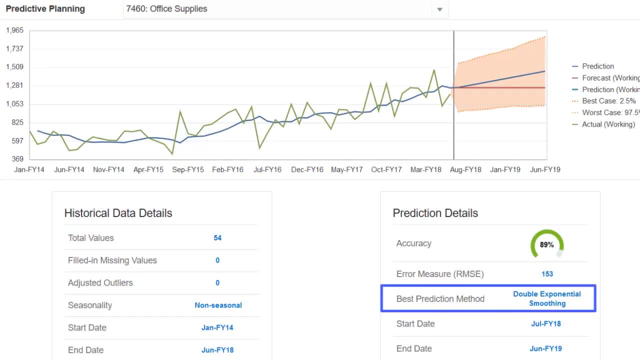 In this example, the Double Exponential Smoothing method is used, resulting in an upward-sloping prediction. This method applies a smoothing technique twice, once to the original data and again to the smoothed data. This method applies a smoothing technique twice, once to the original data and again to the smoothed data. 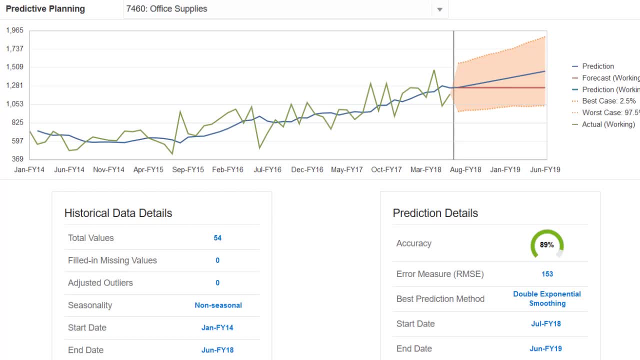 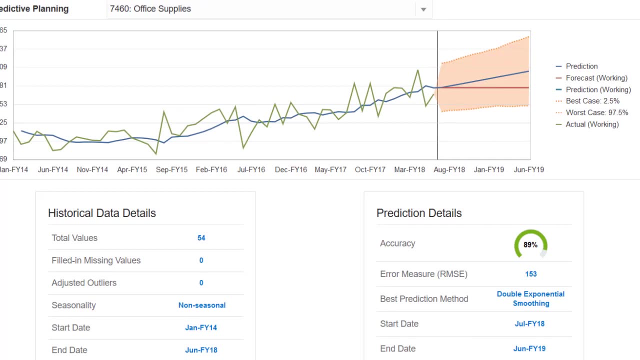 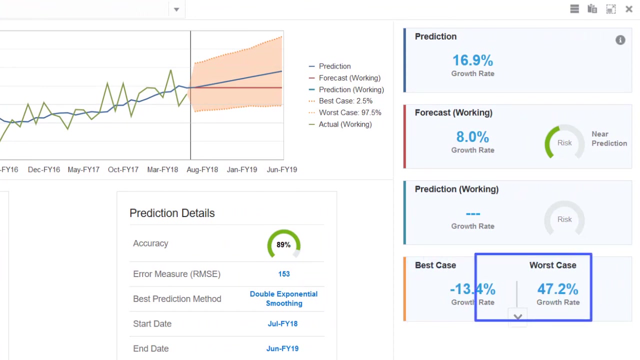 With no discernible pattern in the original data other than the trend, the best prediction will be a sloped line. In addition to forecasting the baseline amount, a prediction interval highlighting the best and worst case scenarios is calculated. The best case is a 13.4% decline in expenses and the worst case is a 47.2% increase. 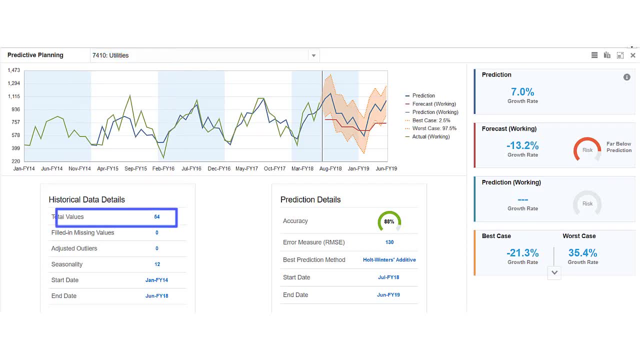 Let's look at the data for utilities. The data appears to be seasonal in nature, with a consistent pattern of peaks and valleys. Each seasonal cycle is shown on the slide. Each seasonal cycle is shown in an alternating blue and white background. The best forecasting method is selected. 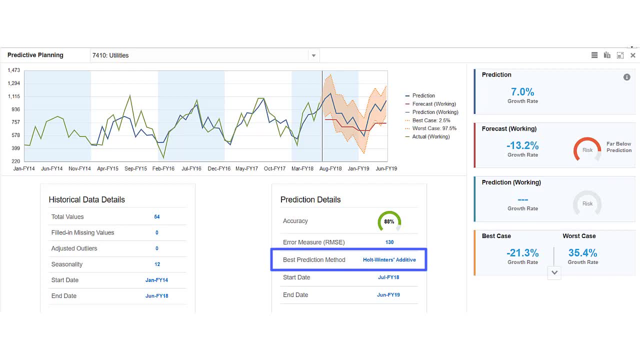 In this example, the Holt-Winters Additive Seasonal method is used. This method follows the pattern of repeating cycles in past data to predict future data. Let's look at telephone expenses. The data doesn't have a consistent seasonal pattern but shows some signs of irregular cycles. 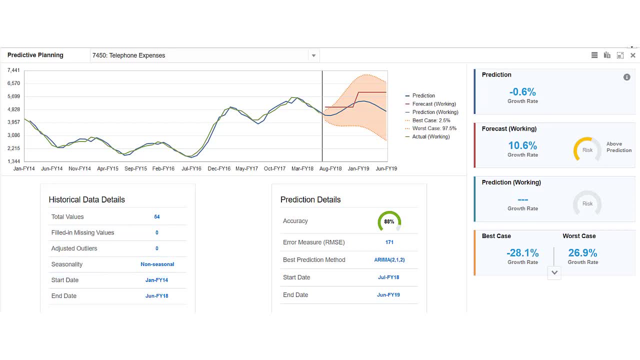 In this case, the historical data doesn't exhibit a consistent trend or seasonality pattern. As a result: predictive planning: selected auto-referencing data to predict future data. As a result: predictive planning: selected auto-referencing data to predict future data. 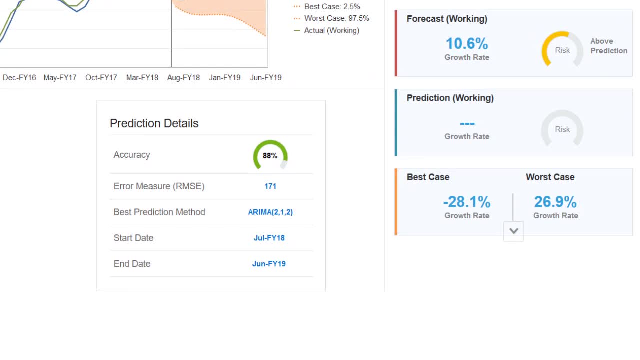 As a result, predictive planning selected auto-referencing data to predict future data, And it selected Autoregressive Integrative Moving Average, or AREMA, a method that uses a blend of forecasting techniques to fit more complex data patterns. There is also a seasonal version of AREMA, named SUREMA, which fits complex seasonal data.